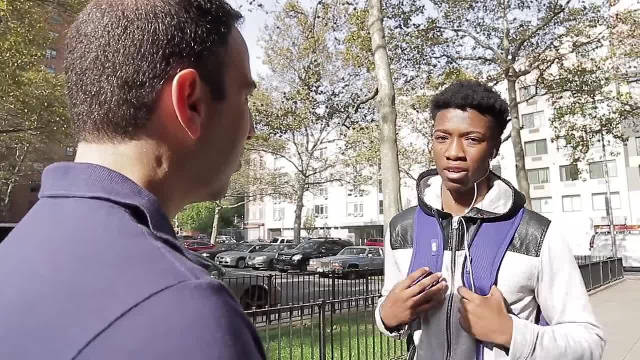 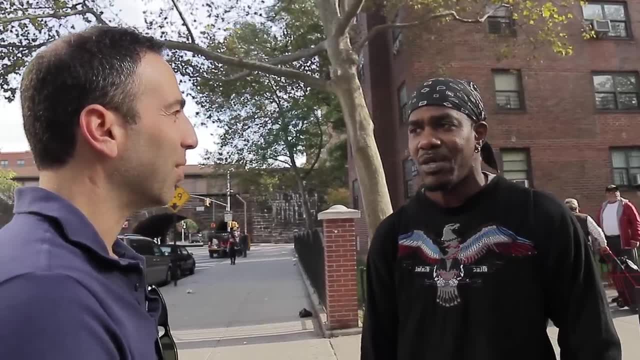 Do you have ID? Yes, Because I have my ID and my friends have their ID, so we know what we need to carry around. Everybody that I know have ID. That's one of the things you need to walk around with New York with an ID. 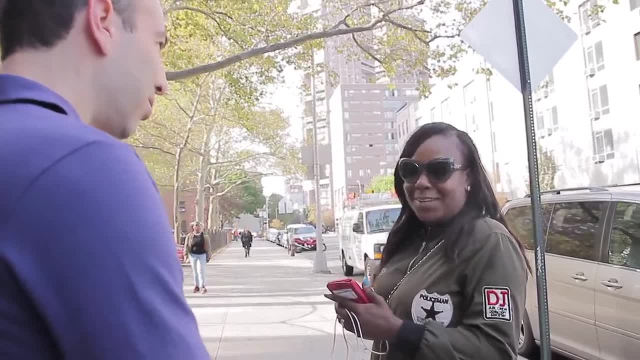 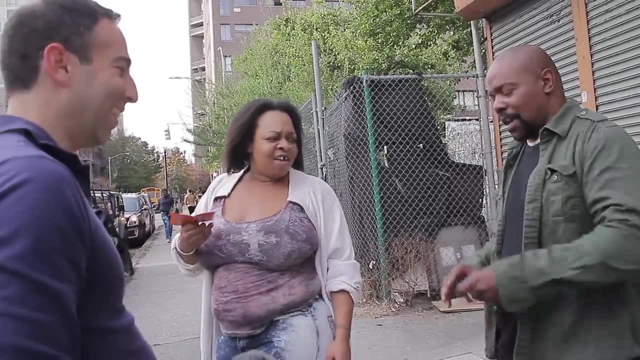 Do you know any black adult who does not have ID? No, I don't. Is it a weird thing to even say that? Yes, it is. What is this? some type of trick candy camera or something like that? I know right, That's the only thing I brought with me. 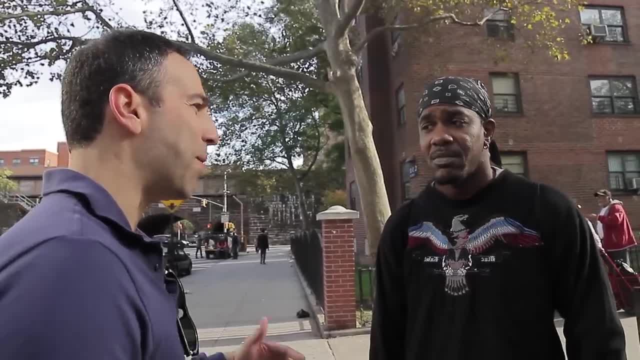 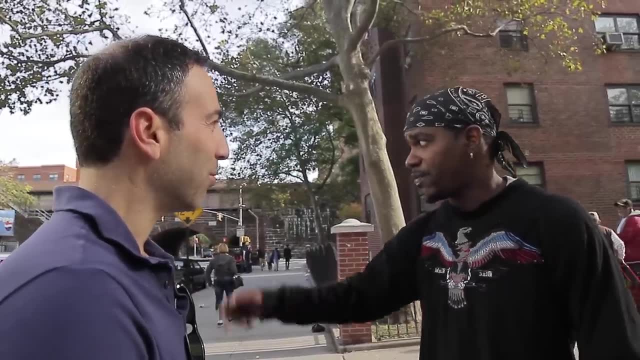 Those are legit IDs. I heard a lot also that black people can't figure out how to get to the DMV. Really, What does that say to you? I know it's that, but I'm 25th year. Do you know where the DMV is around here? 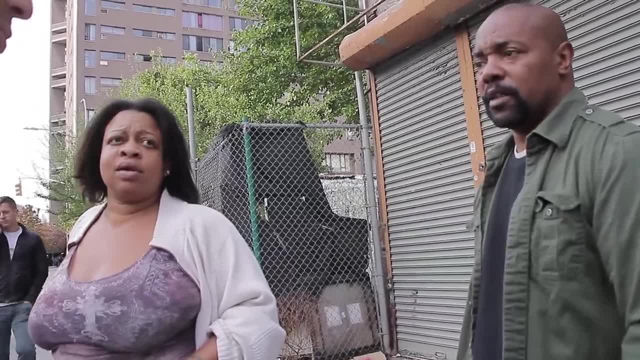 It's on 125th Street and 3rd Avenue. I believe You know how to get there. Yeah, Do you have a problem getting there? if you have to get there? No, I know these sound like silly questions. You know how to get to the DMV. 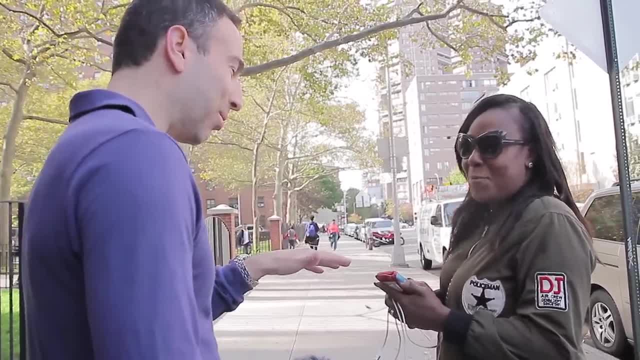 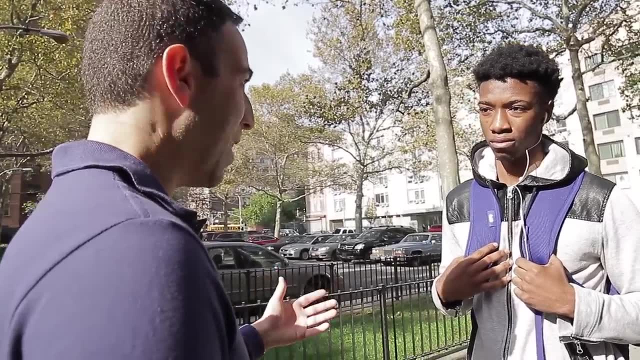 Of course You know where it is. Yes, You can get there. Uh-huh, No problem. No problem, Just checking. Okay, I also heard a lot that black people, especially poor black people, have no access to the internet, can't figure out how to use the internet. 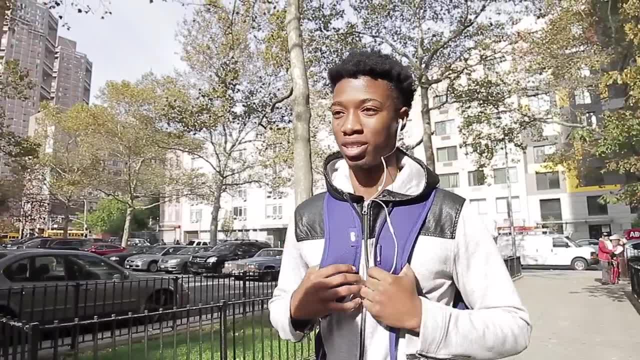 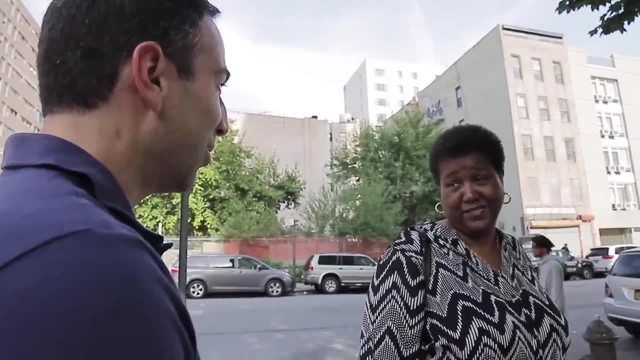 That's just stupidity. honestly, Everybody has access to the internet. Even a little kid can figure out how to work the internet. I've had access to the internet for years. You know how to use it properly. Exactly, I do it at work. 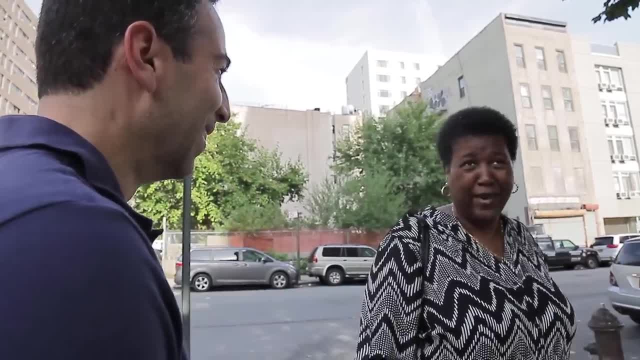 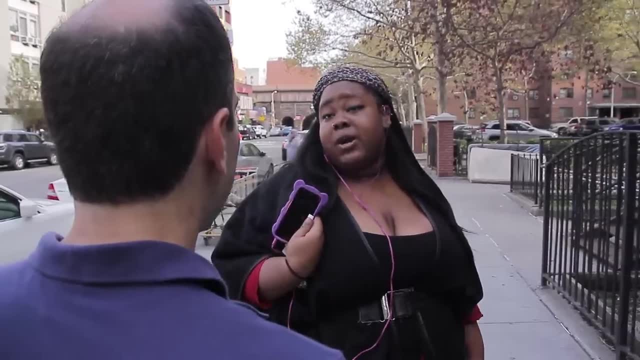 So, of course, I know how to use it. My kids know how to use it. They all have iPads, iPods, whatever. Your phone has data- Unlimited. Unlimited data- Uh-huh, I use my phone as a hotspot. 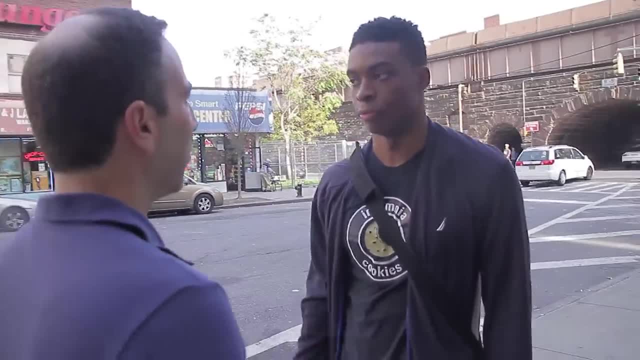 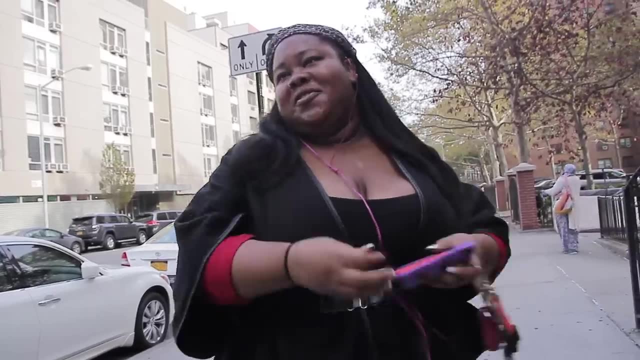 What does that say to you? for the people who have this perception of black people, They're pretty much ignorant of it. That's what my thought process is. I just think that's ignorant. It's ignorant, Ignorant, That's the word I hear a lot. 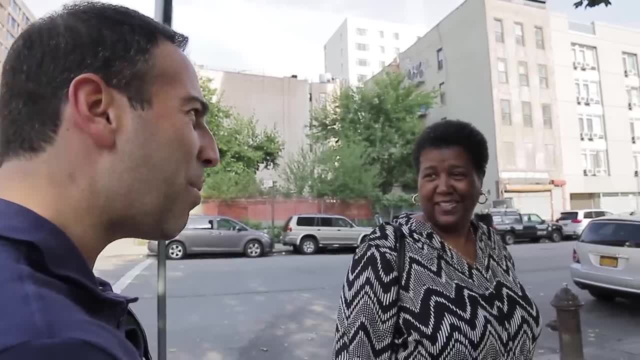 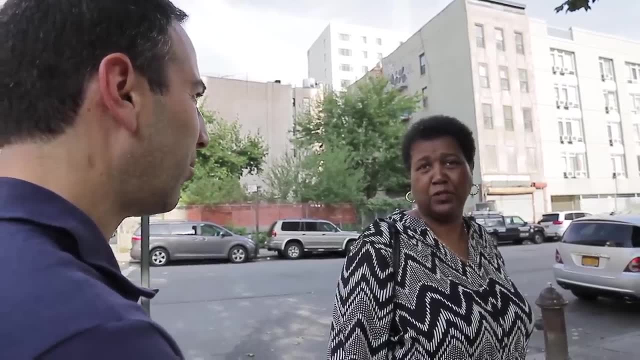 Very, very ignorant. Does it sound racist for somebody to say that? I think it is a little racist, because you know you're putting people in a category and you have no idea what you're talking about. Maybe a little bit of racist in it, but, like I said, I think it's more stupidity and ignorance. 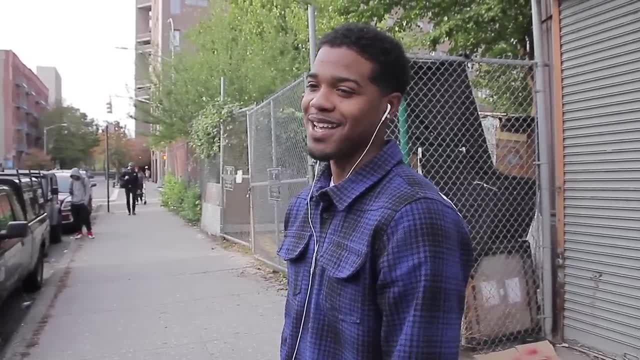 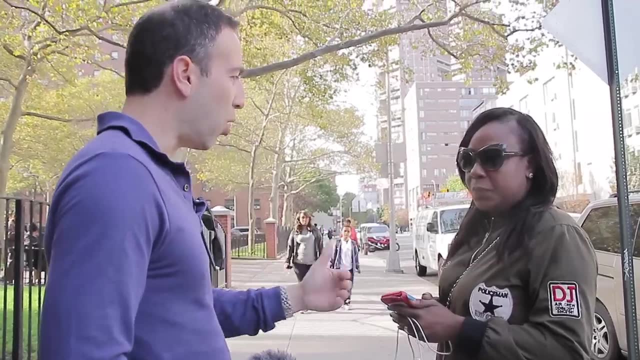 You're judging somebody like: but you're judging somebody because they're black, saying that they don't got it. What people are they talking to? Who are these people talking to? Do you have a problem that if you go to vote and they say, can we please see your ID to?